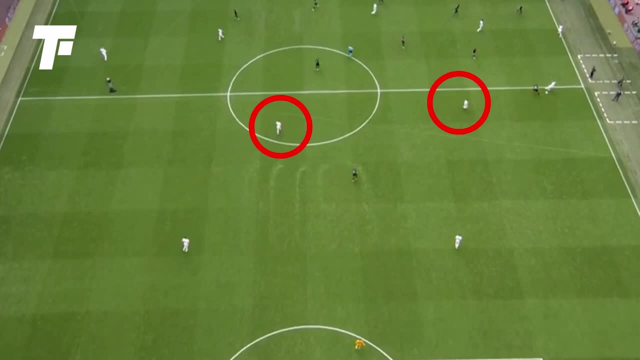 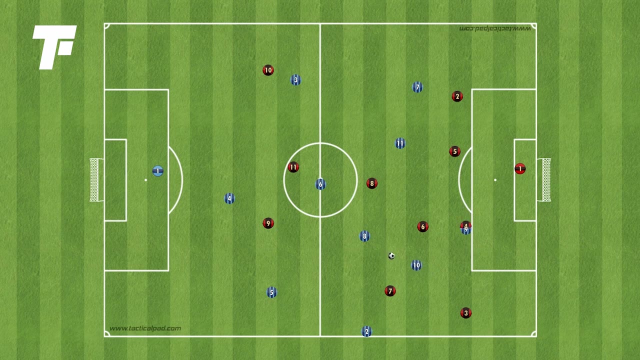 defensive midfielder move during the build-up, Do they drop in? Do they create triangles with the centerbacks or the fullbacks? So now you have to ask yourself what patterns are currently happening, What rotations are currently happening, Anytime that you watch the 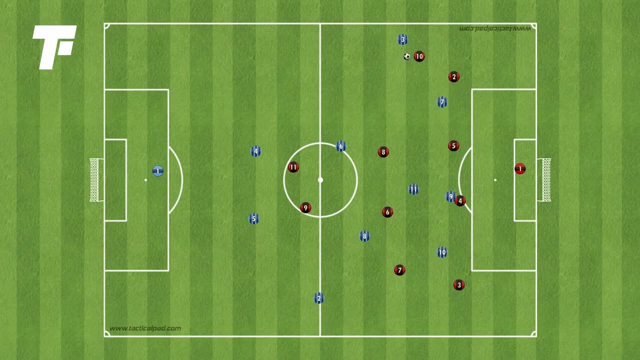 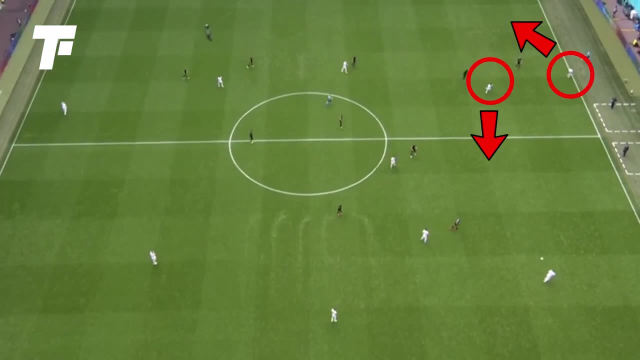 game. you have to identify what patterns are happening to get into the final third. Are they circulating the ball? Are they trying to go forward immediately? Are there any certain rotations that players do often? Who's taking up the half spaces in the build-up and in the 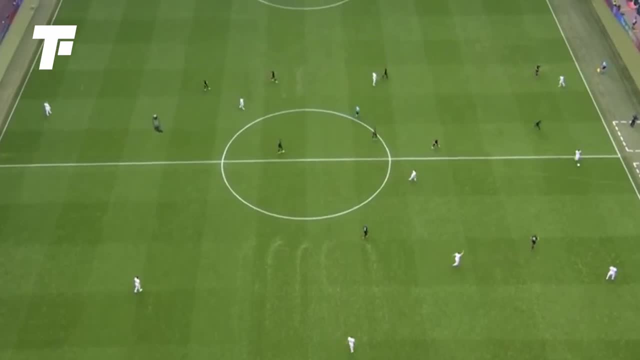 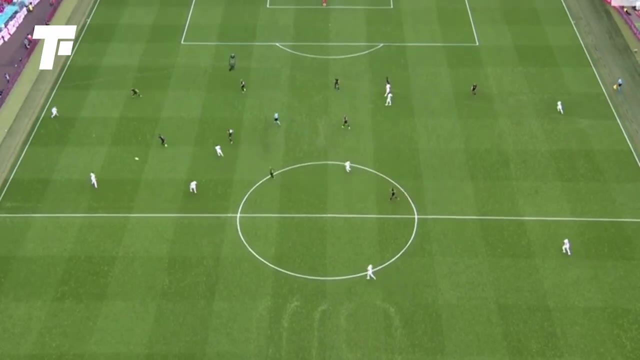 finishing phase. How often does the team look to switch the ball or do they drag out opponents into certain areas? So notice how, in this sequence, they are moving the ball side to side. They notice that on the left side it's a little bit congested. They can't. 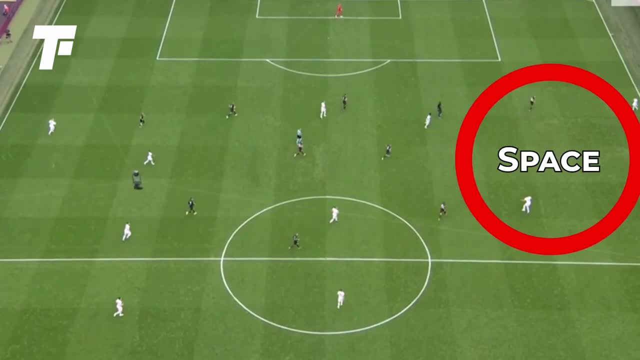 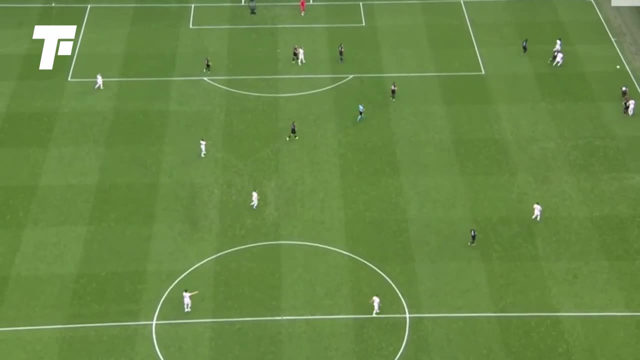 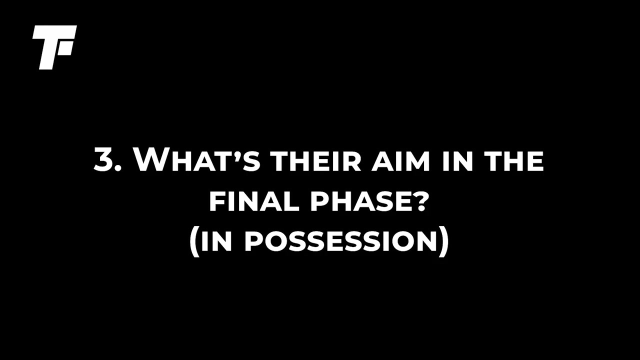 get anything done in that area, So they quickly rotate the ball to try and attempt to create something. on the right side, Two players are making the run in deep. They're able to progress the ball in that area and draw the foul. And lastly, what is the team's aim during? 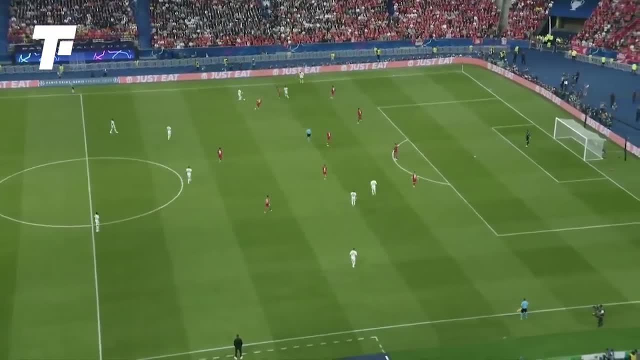 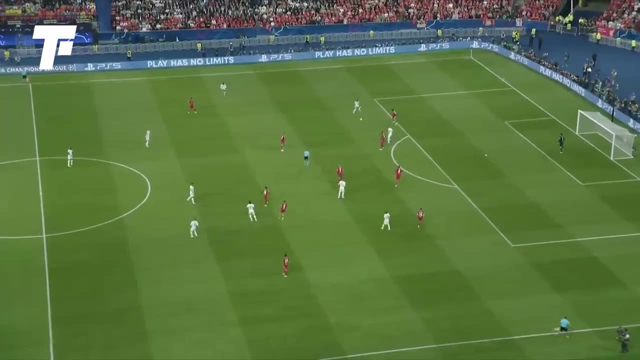 the final phase. In this clip right here you can see how this team is rotating the ball side to side. They switch play at least two or three times, trying to find that isolation, with the players out wide either for a 1v1 or a 2v1 situation. In this next clip you can see: 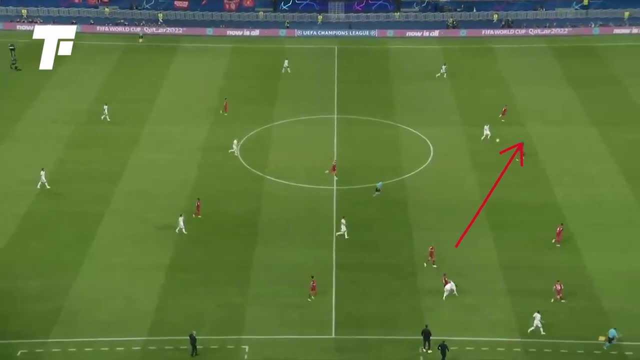 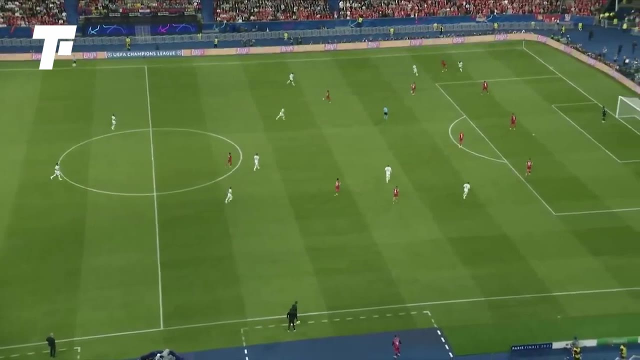 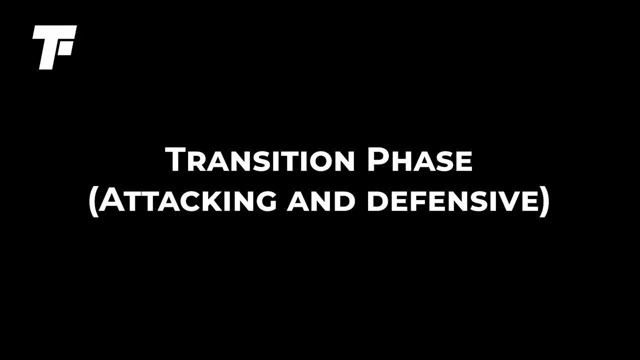 the same exact thing happening: Big long switch to create that one-on-one chance and try to create an attacking opportunity. Just like you see here, they're able to try and create something inside the box. They're able to win a corner kick. Now, during the transition phase, you want to identify. 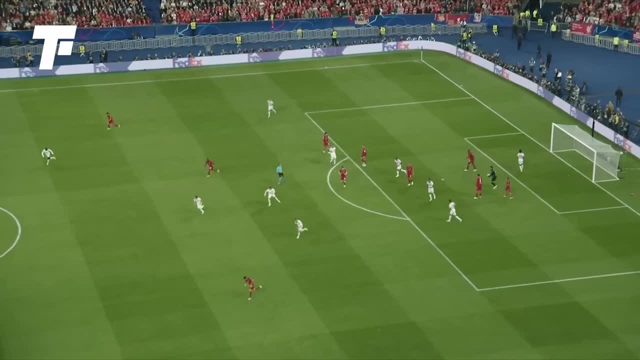 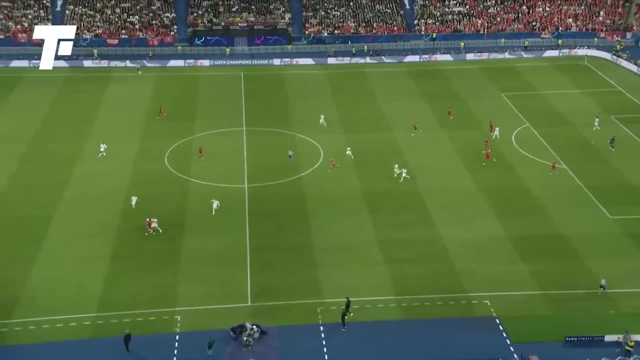 what are the players' reaction and how does the team react as a whole? Are they keen to win the ball back right away? Are they just dropping in back into formation? When they win the ball back, do they look to counterattack quickly? Are they looking? 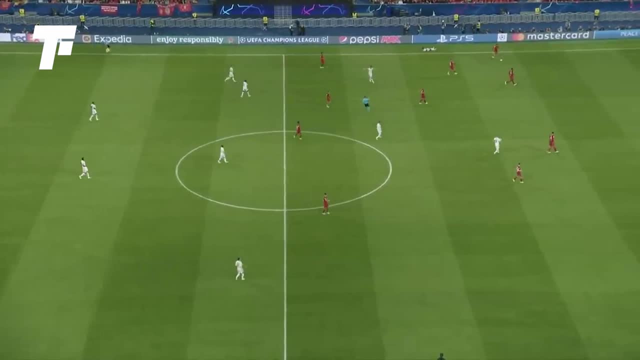 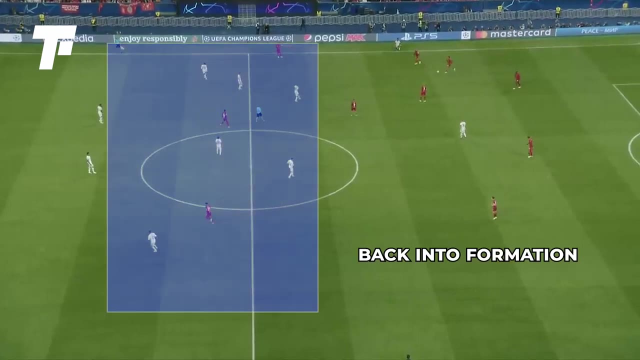 to circulate the ball. What is their reaction when they are in that transition? So, for example, in that clip before you saw how right away the offensive team looked to counterattack and then the defending team look to drop back. Here you can see how the